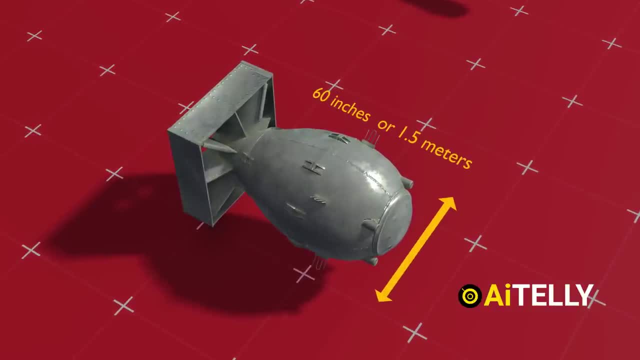 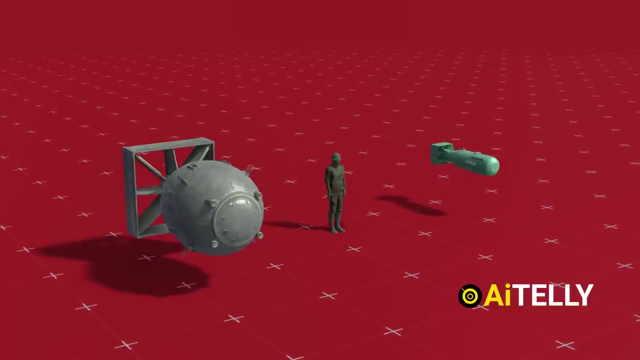 meters, but a much larger diameter of 60 inches or 1.5 meters. Comparing this to a person will help you understand its size Even better. let's compare this to this classic American SUV, as you see, both of the nuclear weapons look small considering the amount of destructive. 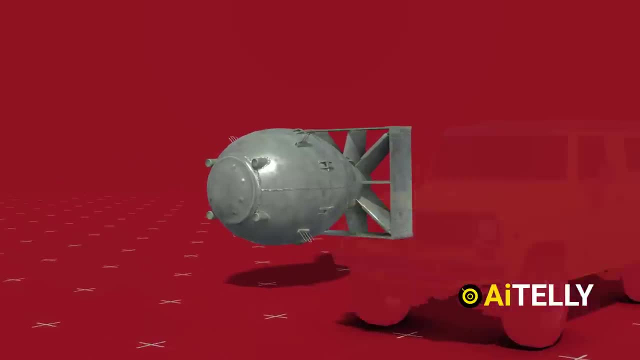 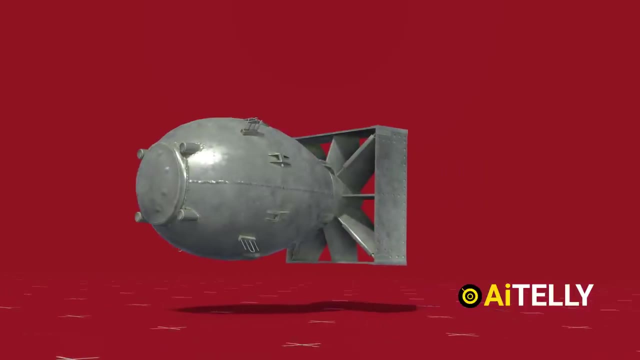 power packed into it. This nuclear weapon weighs around 4,800 pounds and is the largest nuclear weapon in the United States. The Fat Man atomic bomb is a large, heavy plutonium imploded using the same charges as the Little Boy, While the Little Boy is the name suggests. 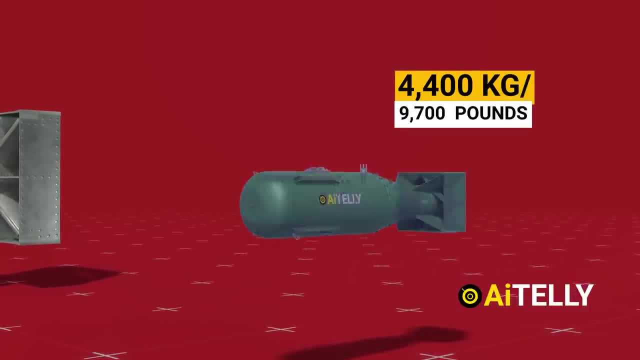 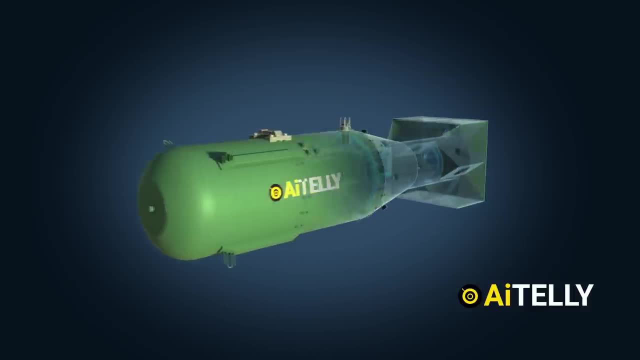 weighs just shy of 4,400 kilograms or 9,700 pounds. Before we dive into how this works, we have to understand the parts of the nuclear weapon Starting from the back. these are the box-tail fins meant to stabilize the bomb. 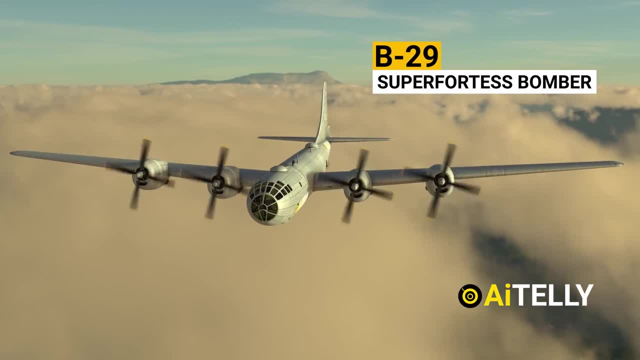 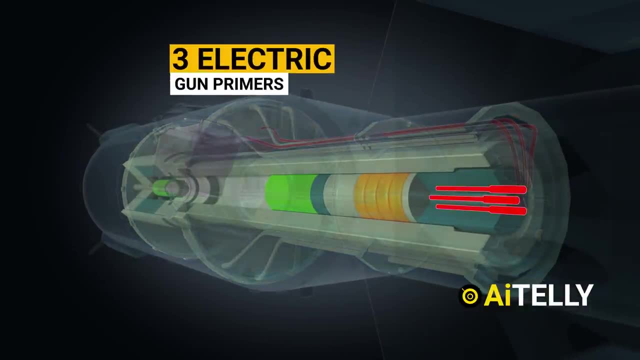 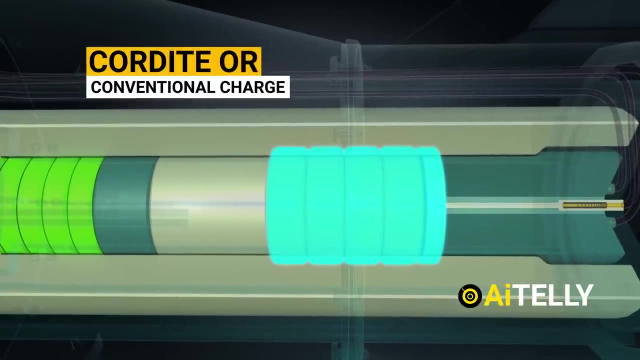 What dropped from this B-29 Superfortis bomber. So These are the three electric gun primers. The primer is the device responsible for initiating the propellant combustion located here also known as the chordate or conventional charge that will push this projectile at an explosive. 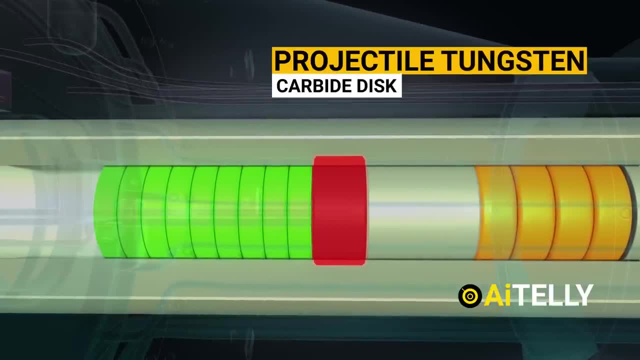 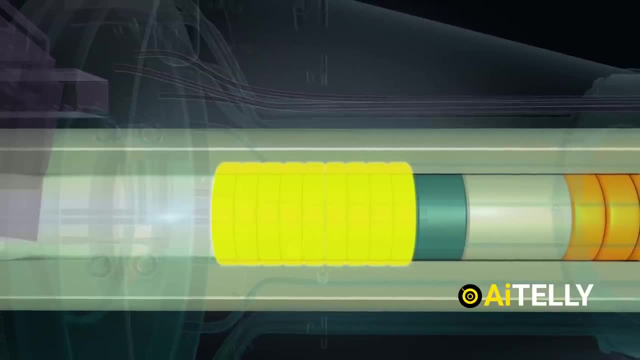 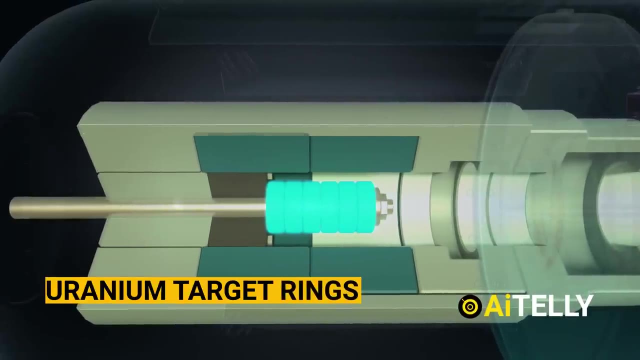 force Moving ahead. this is the projectile tungsten carbide disc And the most important part is the uranium-235 hollow projectile rings. It weighs around 84 pounds or 38.4 kilograms, While the front is the uranium target rings that weigh around 56.2 pounds or 25.6 kilograms. 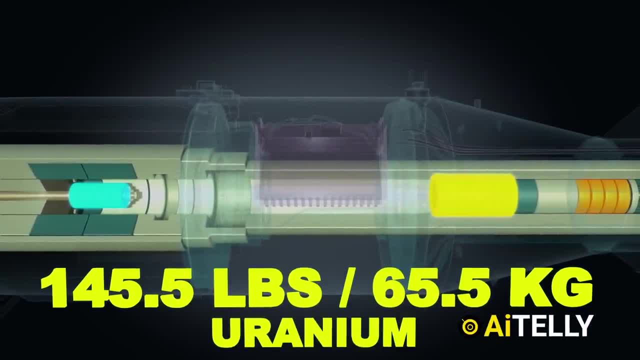 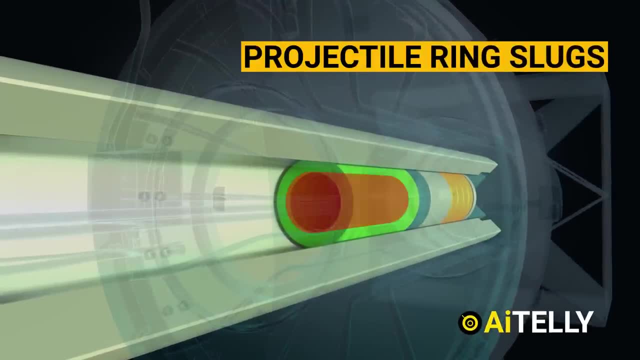 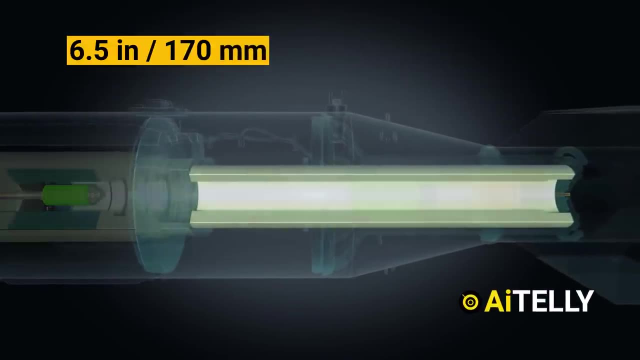 That is around 145.5 pounds or 65.5 kilograms of uranium. Closely note, as it is very important to understand. the projectile ring slugs are hollowed and designed for the target rings to enter. All these mechanism and parts are encased in a 6.5 inch or 170 millimeter smoothbore. 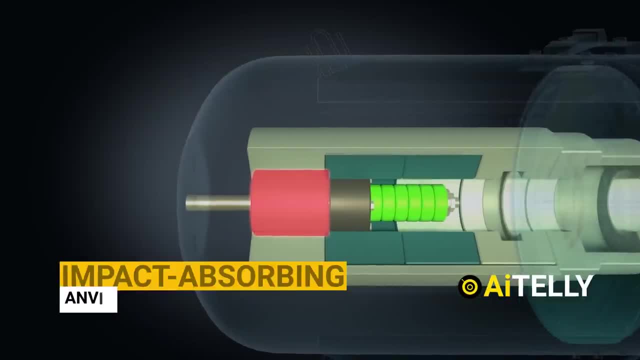 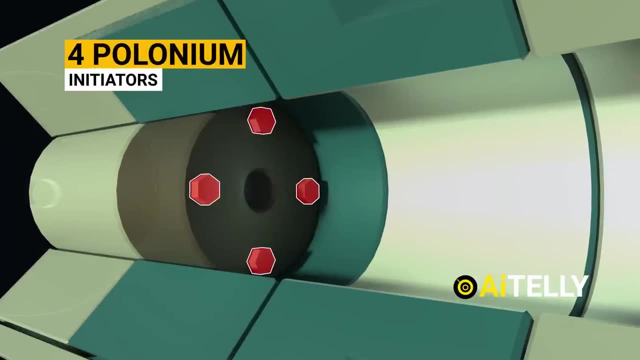 gun barrel Moving to the front. this is the impact absorbing anvil. Just above it is the tungsten carbide plug. These are the four polonium initiators placed on the tungsten carbide. They are kept to make sure there will be a nuclear chain reaction when it is dropped. 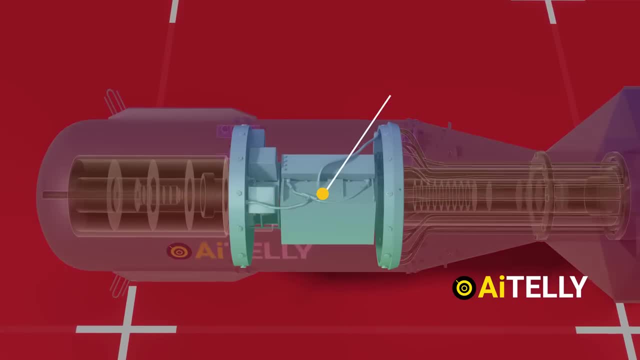 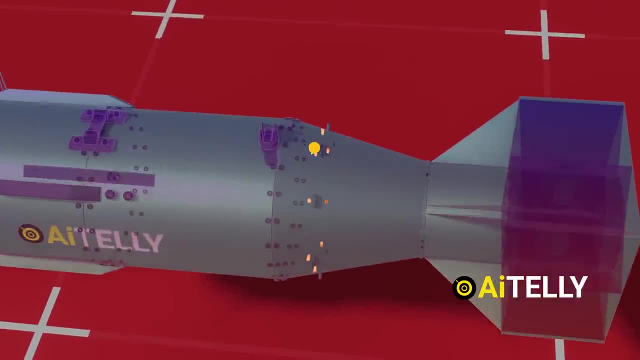 and activated. Moving to the top of the structure are the arming and fusing equipment. Let's move outside this atomic bomb to understand it better. These are the barometric sensing ports and manifolds. The barometer helps to identify the altitude of the bomb. 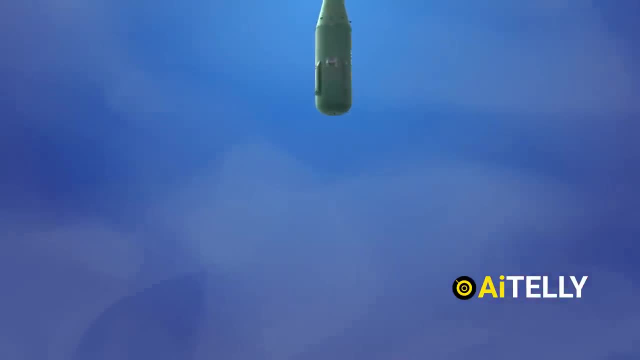 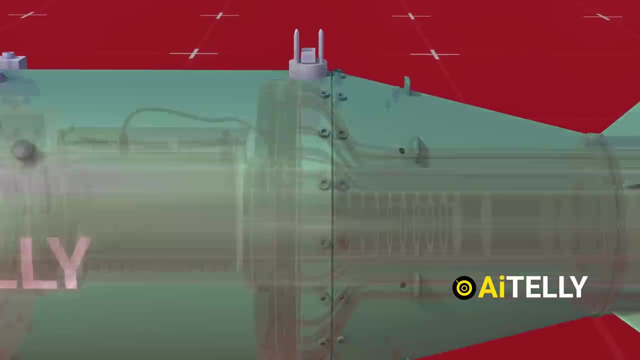 It is located at an altitude in which the bomb is located so that it can activate this archy fusing radar altimeter, which is these curvy looking objects that activates before reaching the ground. Just above it is the electric plug, and some refer to this as the arming wires. 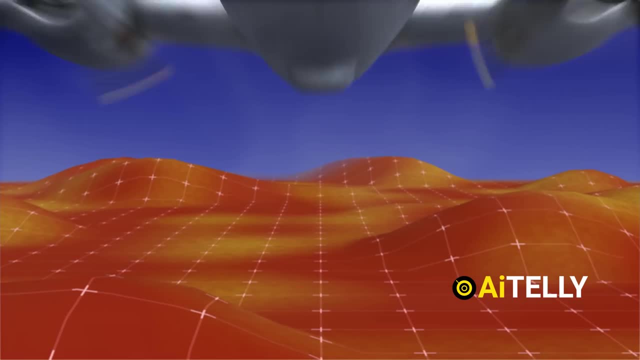 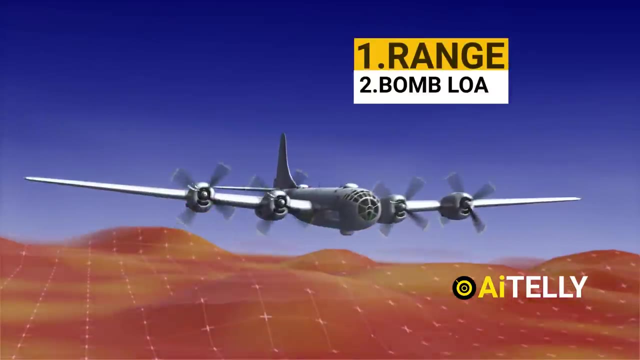 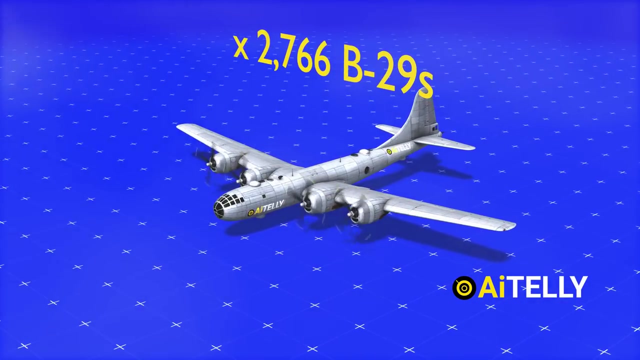 All that destructive power requires a platform to transport this nuclear weapon. The answer is this B-29 Superfortress. It was also the world's heaviest production plane because of increases in range, bomb load and defensive requirements. Boeing built a total of 2,766 B-29 Superfortress planes and it was the most advanced four-propeller. 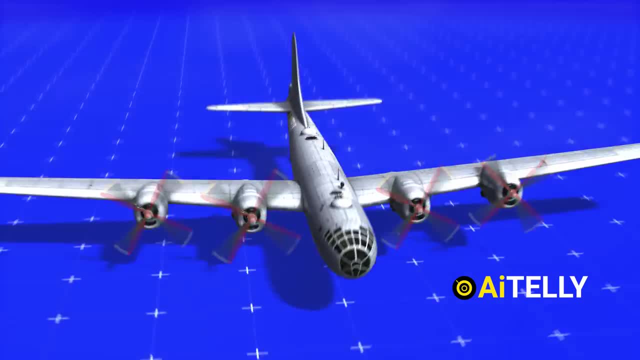 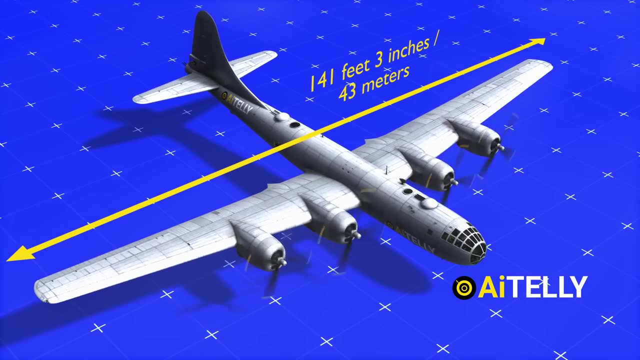 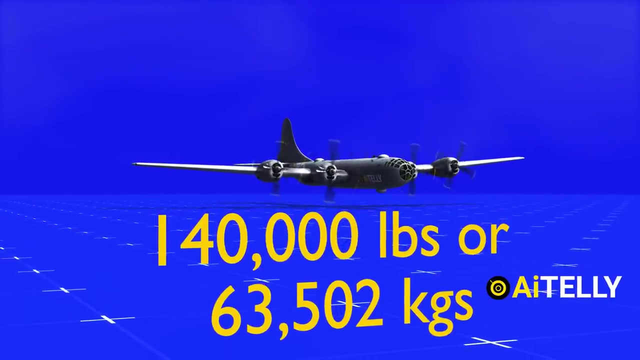 driven bomber of the Second World War. It has a length of 99 feet, or 30.1 meters, with a huge span of around 141 feet 3 inches, or 43 meters. Interestingly, the plane has a gross weight of around 140,000 pounds, or 63,502 kilograms. 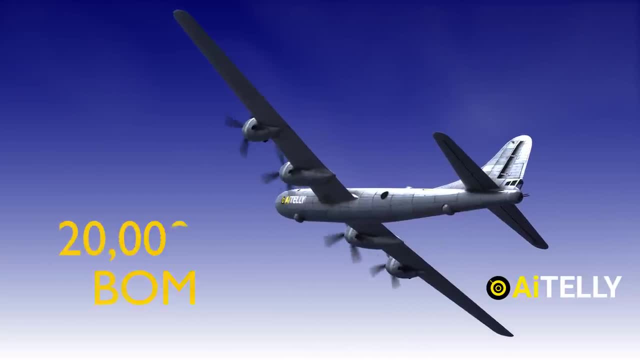 and could carry a 20,000-pound weight. This means that it can carry a total of 1,000,000 pounds or 1,500,000 kilograms. This means that it can carry a total of 1,000,000 pounds or 1,500,000 kilograms and could carry a 20,000-pound weight. 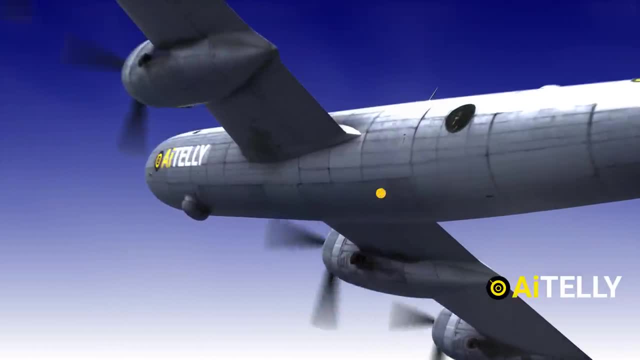 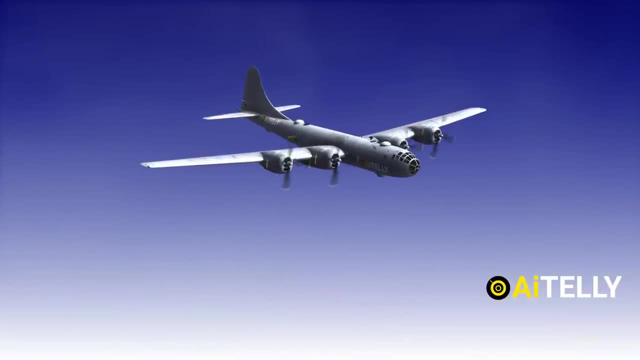 The bomb bay door is located just below the fuselage and it can open them as shown in the animations. As stated, this is one of the most fortified plane in that era. It can carry around 12, 50 caliber machine guns and remote-controlled turrets, as shown. 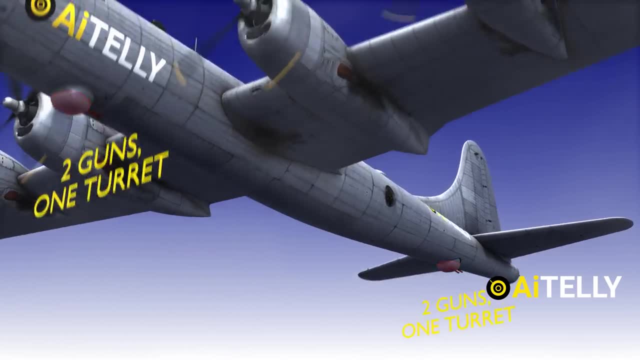 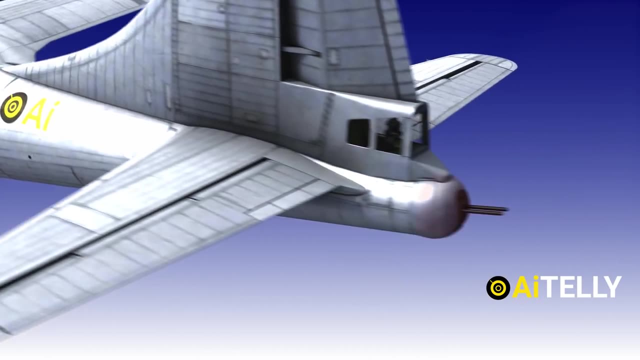 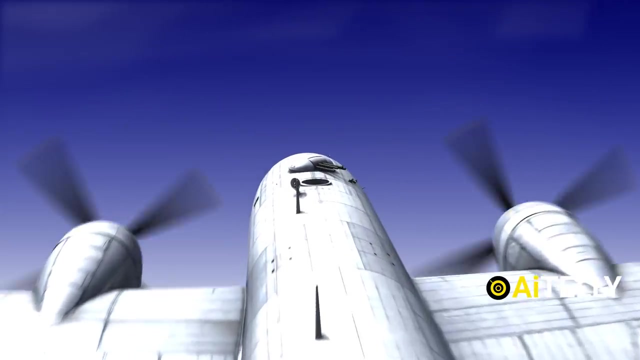 in the animation: Two below the plane, four above the fuselage, two remote-controlled turret, one above and below, near the tail, And the last two are located at the back of the plane. And that is one protected gunship. Now that we've established the B-29's superfortress as a primary transport, let's take a look. 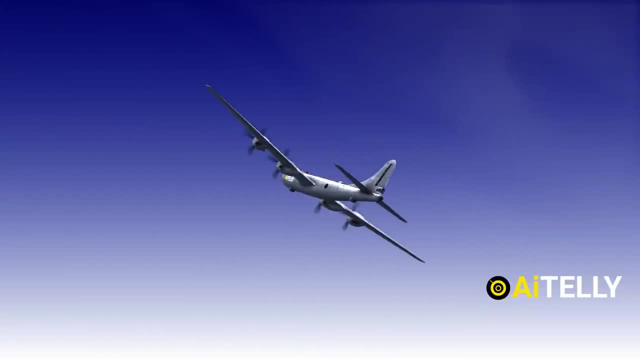 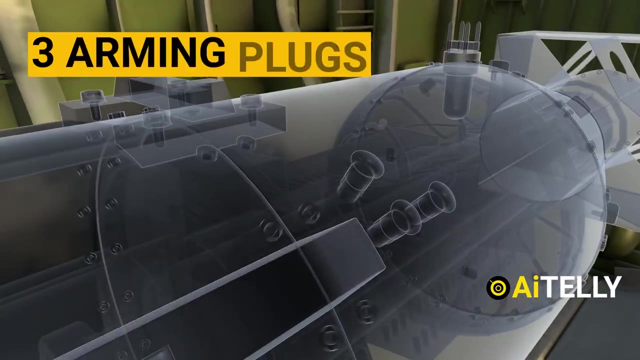 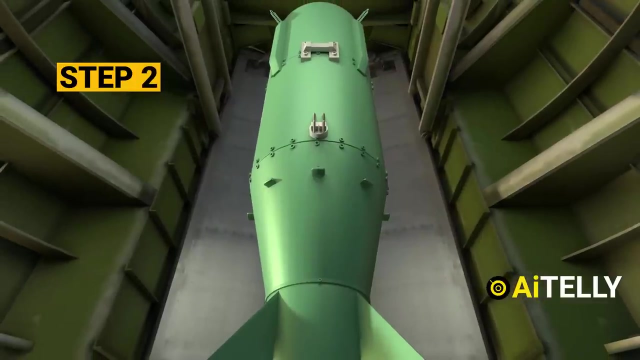 at how this nuclear bomb works in basic step-by-step format. Step number one: Before opening the bomb bay doors, all three arming plugs are pulled, one after the other, by the weaponer, William Sterling, Deke Parsons. Step number two: The door is opened and the bomb falls due to gravity. 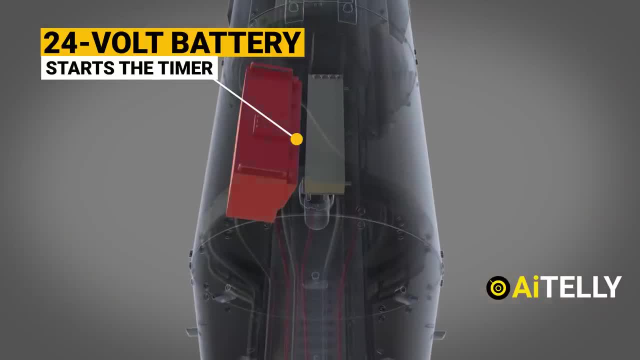 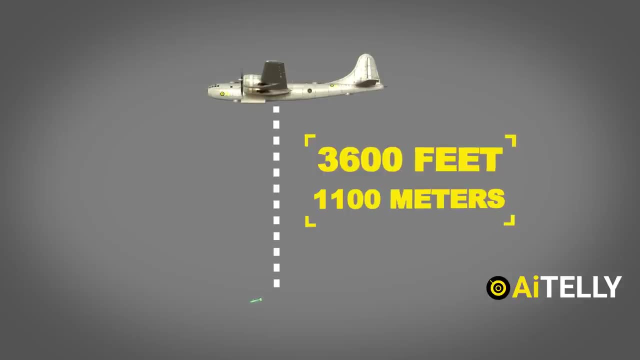 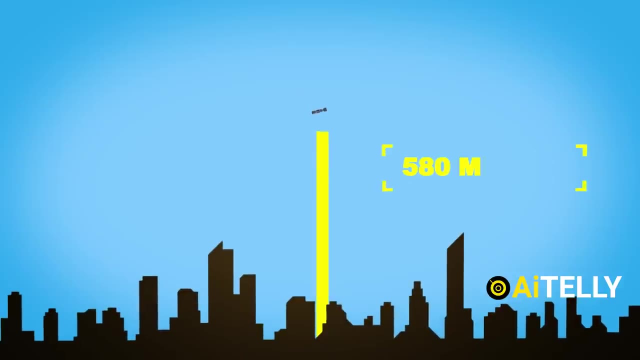 Then it switches to its internal 24-volt battery and starts the timer After 15 seconds. the bomb would be approximately 3,600 feet, or 1,100 meters, away from the aircraft. Step number three: The barometer senses the desired height of around 580 meters or 1,900 feet. 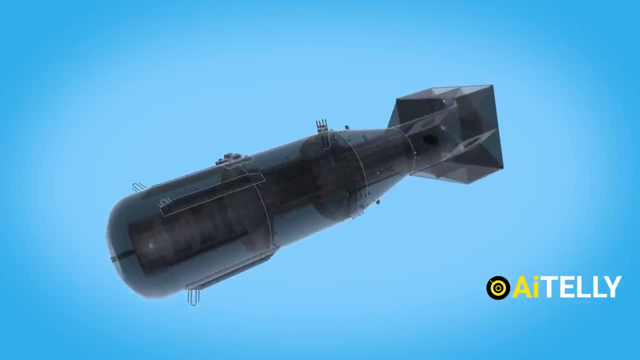 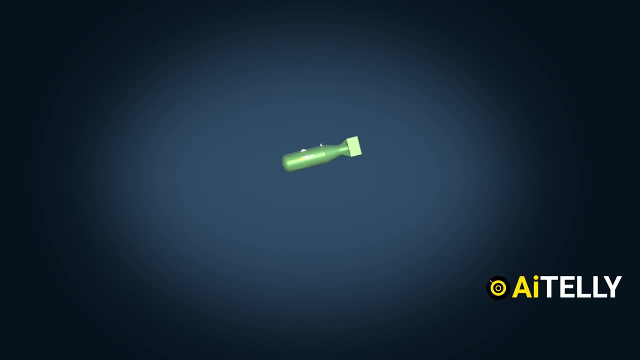 As the little boy was designed to be an airburst above the ground, The membrane closed a circuit activating the multiple radar altimeters located at the front of the bombs. The barometric stage was added because of a worry that external radar signals might detonate the weapon too early. 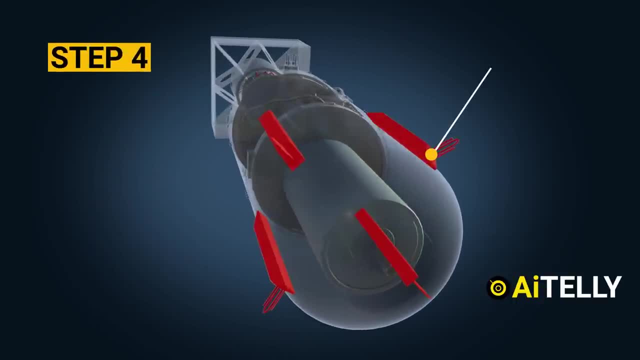 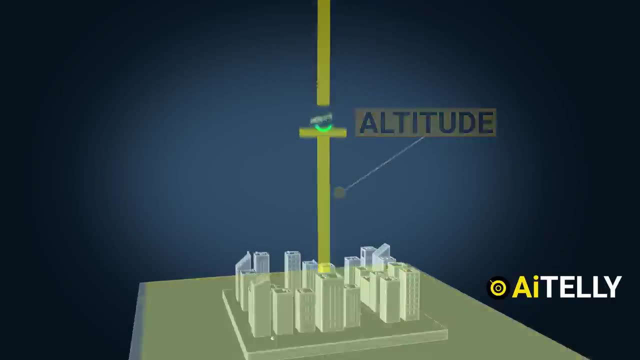 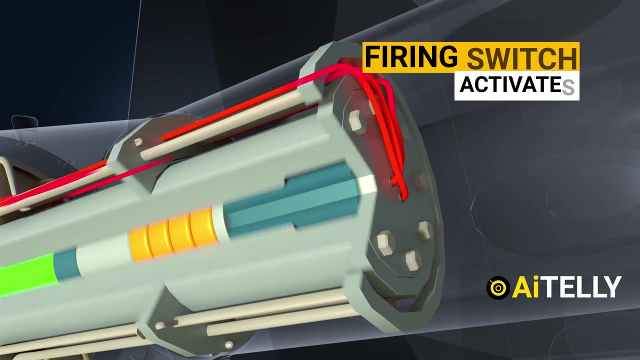 Step number four: To ensure accurate detection of final altitude, multiple radar altimeters were utilized. This process involves measuring the altitude above the ground, beneath the aircraft or the little boy, through the timing of radio waves travel reflection and return. Once the correct height was sensed, the firing switch activates. 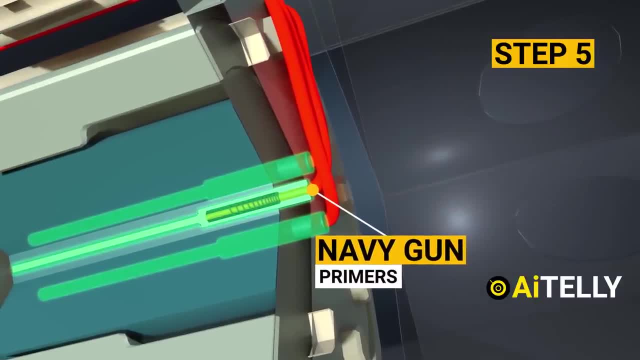 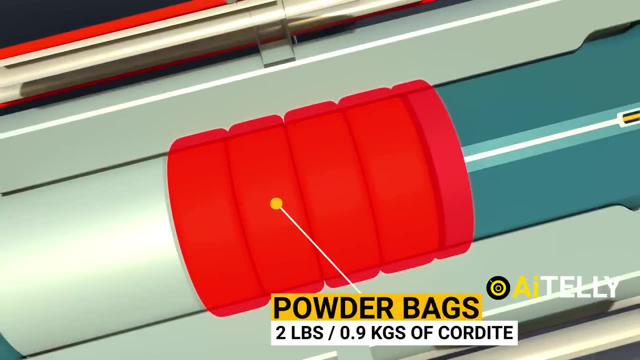 Step number five: This ignites the three Navy gun primers in the breech plug. Step number six: This sets off the charge consisting of four silk powder bags each containing two pounds or 0.9 kilograms of cordite. Step number seven: 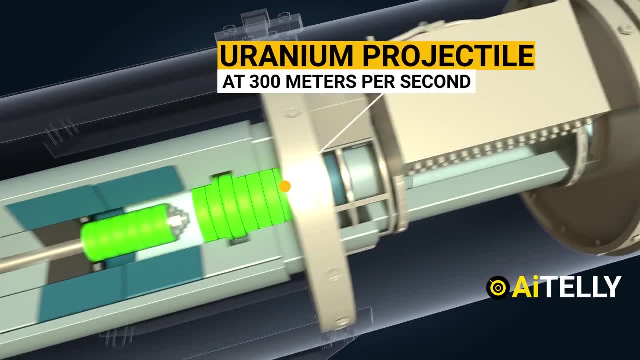 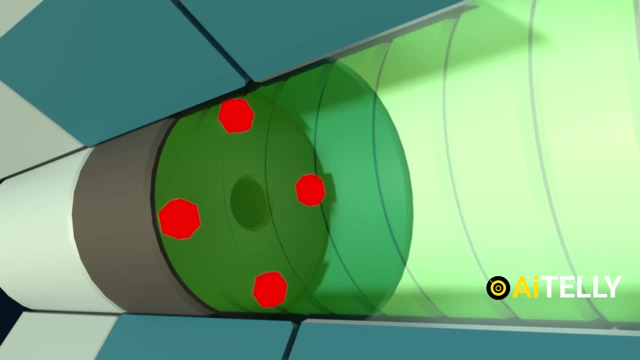 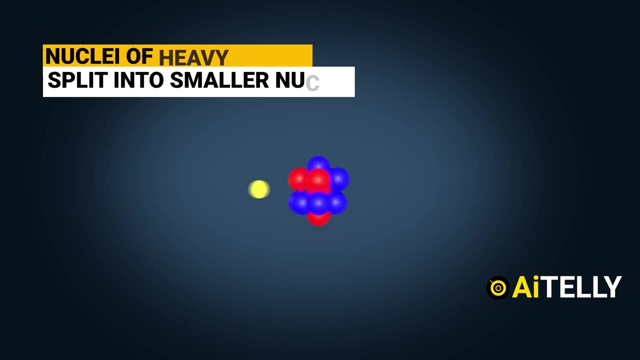 The uranium projectile will be launched at 300 meters per second toward the opposite end of the gun barrel. Step number eight: Four polonium initiators placed on the tungsten carbide initiate the nuclear reactions. Step number nine. Step number eight: fission happens. The nuclei of certain heavy atoms split into smaller lighter. 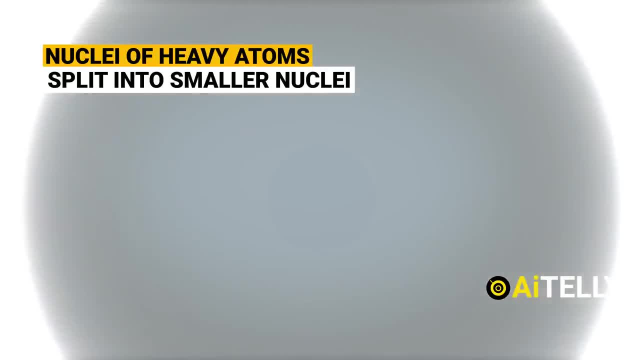 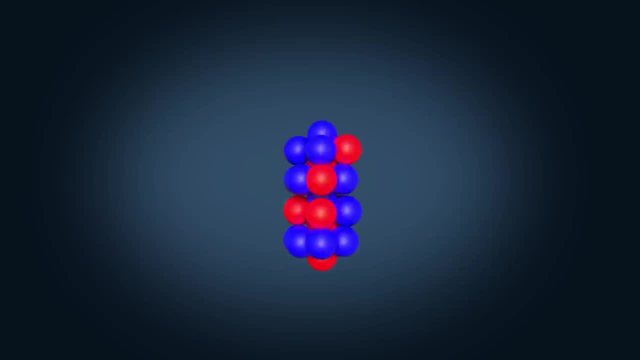 nuclei, releasing excess energy in the process. Let's dive a little bit deeper. The neutron strikes the nucleus and is absorbed. The absorbed neutron causes the nucleus to undergo deformation. The nucleus fission releases an average of two or three neutrons, thus creating a chain reaction or, in some words, an.